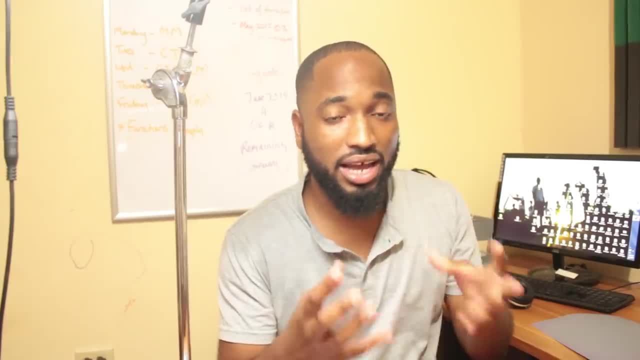 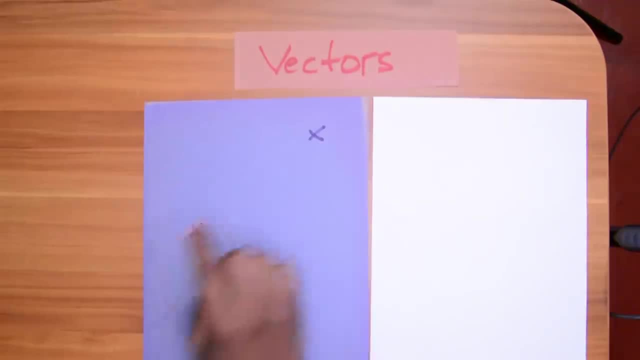 so this video. I just want to take some time to conceptualize and generate the idea of how you should be thinking when you think of vectors. right, let's suppose we have two points and I name these points and I name these points a and b. let me just darken up those points a and b. 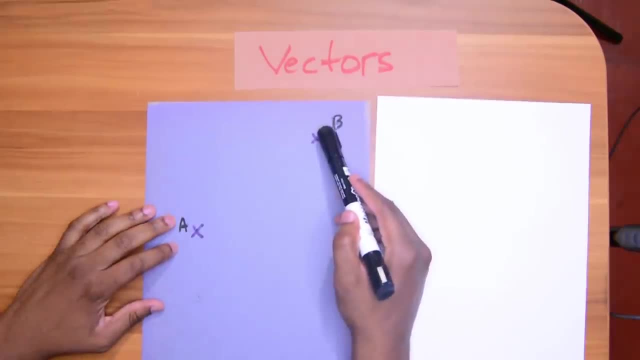 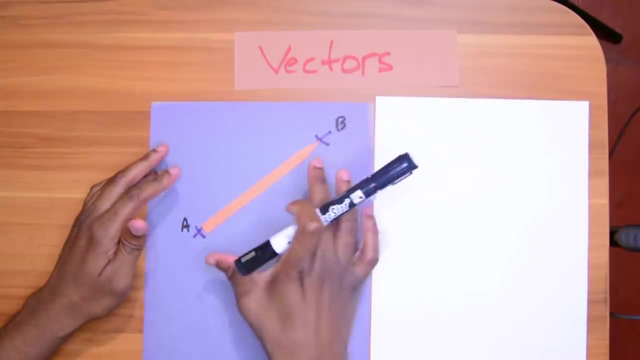 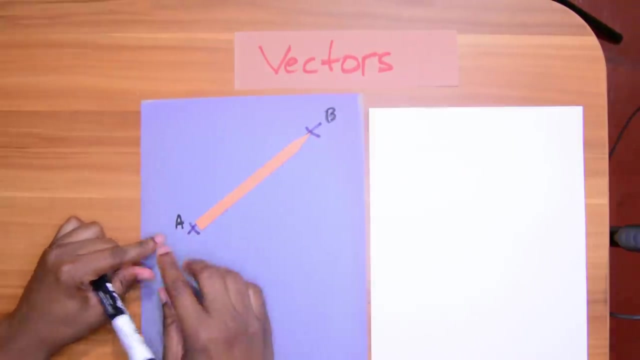 if I want to travel this along from a to b, that is a vector. so a vector is just a directed line, segment, piece of a line in a direction from a to b. and let's say, to go from a to b I will have to go across here. this is looking at it from the x. 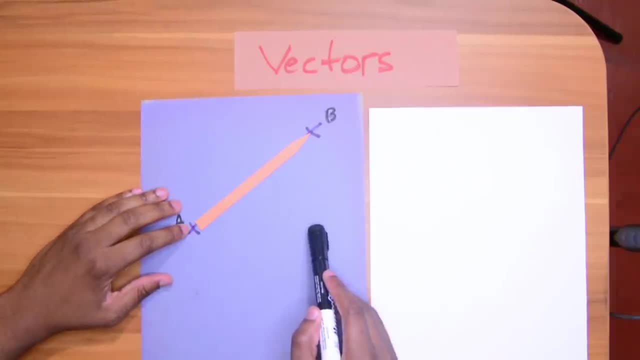 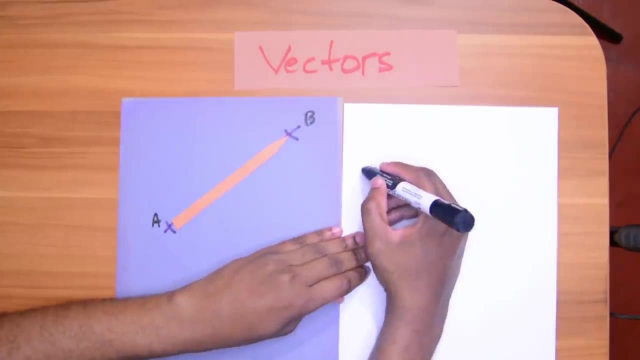 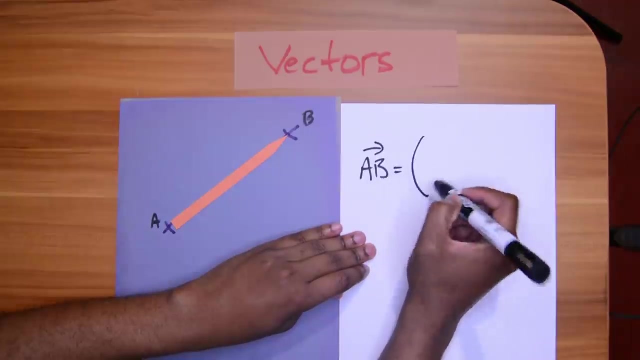 So the horizontal I'll have to go across, let's say, 4, and then go up 3, or let's say I go across 5 and then go up 4.. That means AB, and this is how we write vectors. AB from A to B arrow is equal to 5, 4.. 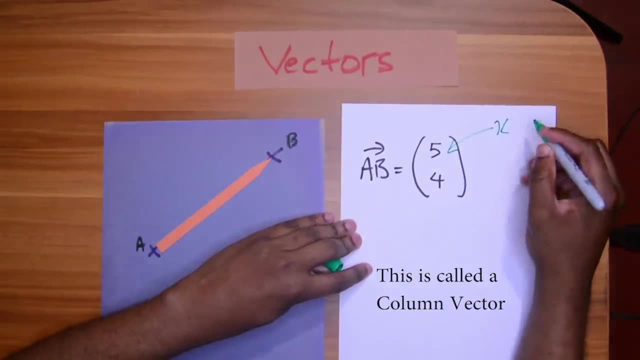 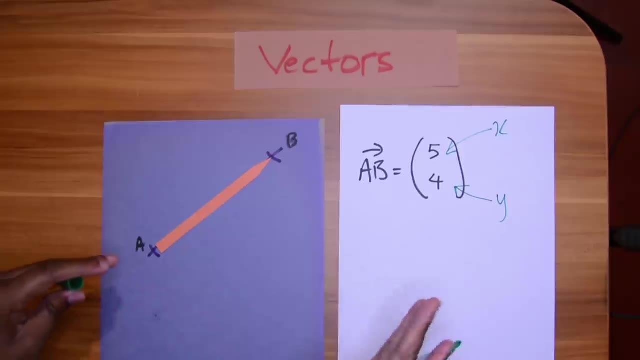 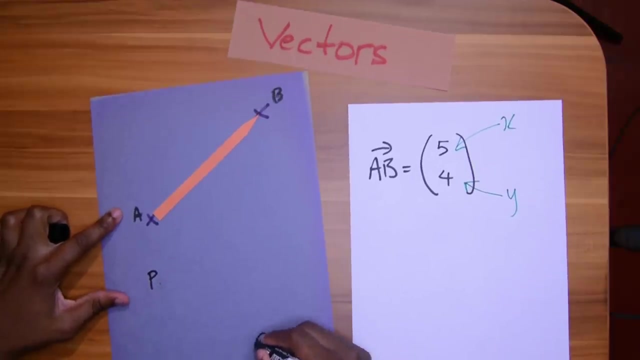 So in this format, the 5 here represents the x value and the 4 here represents the y value. So the x is how much we move horizontally and the y is how much we move vertically. Now if I created another point, let's say maybe P and Q, and I said I want to go from P to Q. 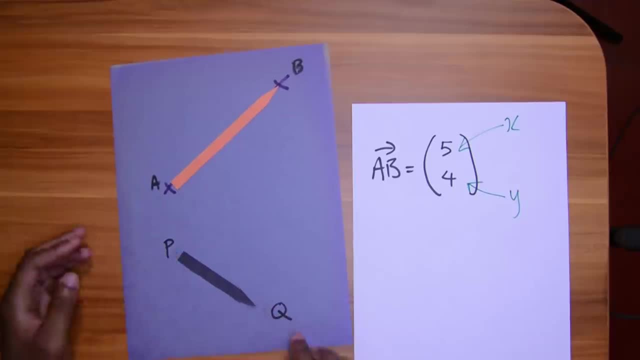 then I could come out with the next vector, P to Q, and maybe I'll have Q here and P here, So that vector looks like that P to Q. Now you'll notice that this vector still goes across. so this vector still may be going across. we'll say vector PQ. 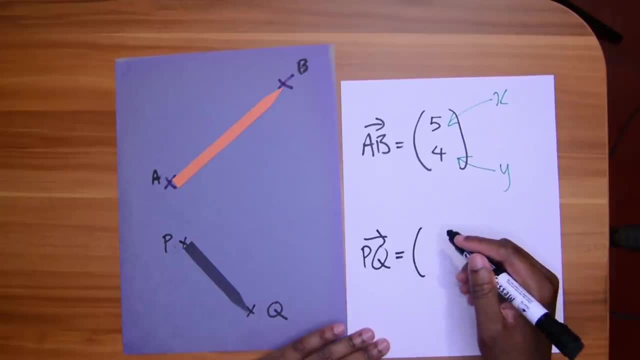 let's let him go across one number you've seen- I feel you know you're seeing 2, and let him go down 3.. Now the problem is it's going down. so if it's going down, we have to indicate that. 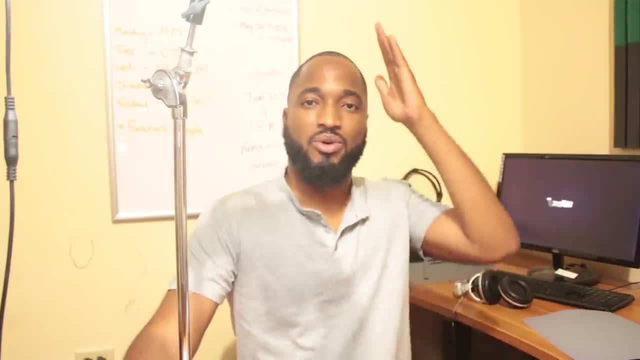 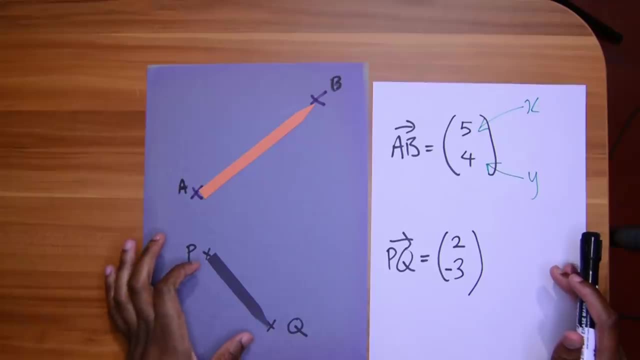 If you're going to the left or going down, we'll put a negative sign. Now, the very important thing about vectors- and physics people you may know about this- is vectors include a matrix, So this one has a magnitude. like you see, this one is small, so he's a little smaller magnitude. 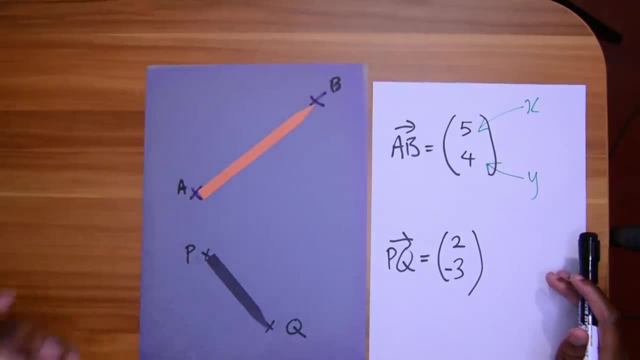 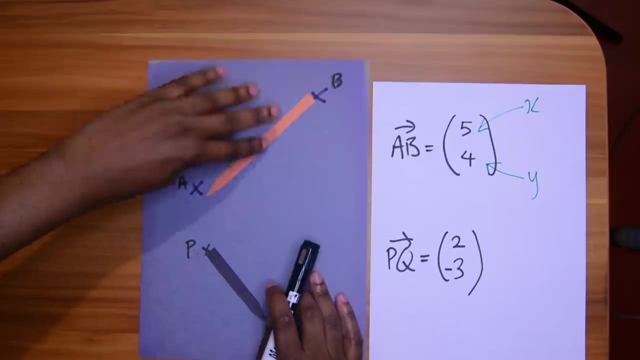 this one is big, so he has a bigger magnitude, but it also includes a direction. For example, if I turn this around like this, this is not vector AB anymore, this is vector BA, But if I turn it back around, it's vector AB. 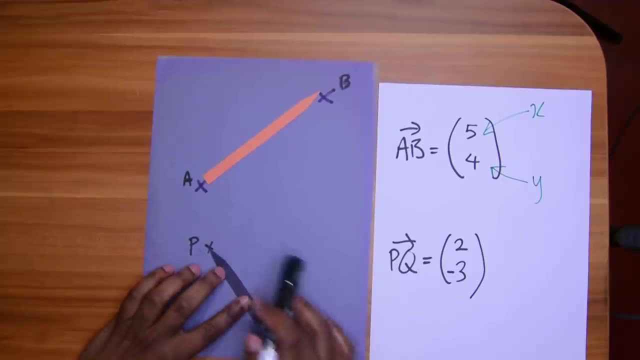 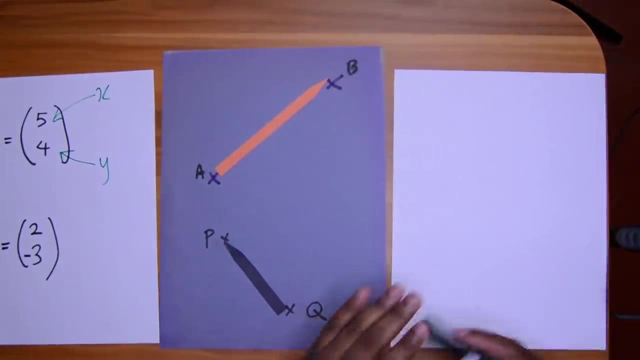 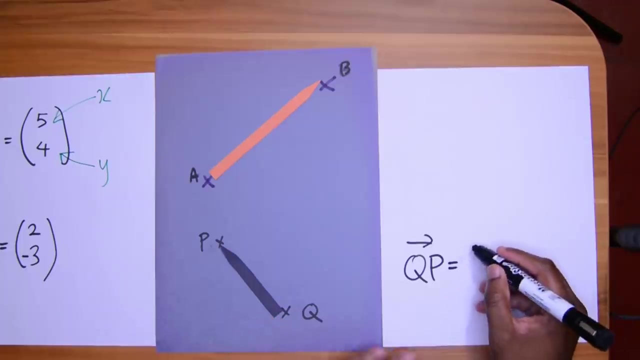 How about? if I turn around this one? this becomes vector QP. Let's see what vector QP will be. Vector QP would mean that I I'm going to the left 2 units and I'm going up 3.. 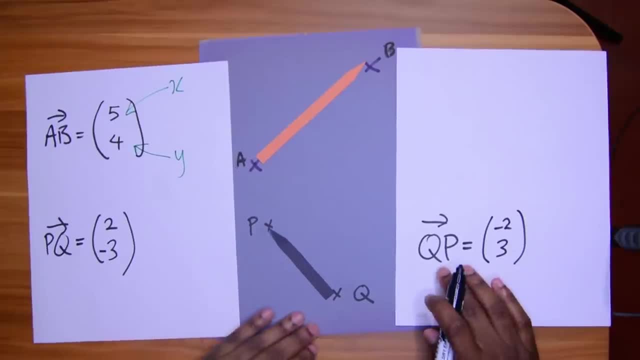 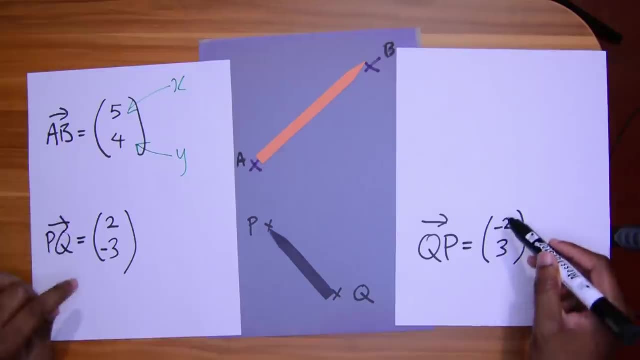 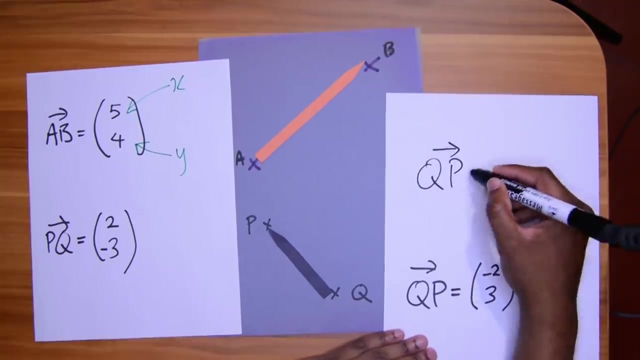 Now, if you compare, now if you compare QP with PQ, you'll notice a little something happening there. It's the negative inverse, the additive inverse. So we can actually write stuff like this: QP is equal to negative PQ. 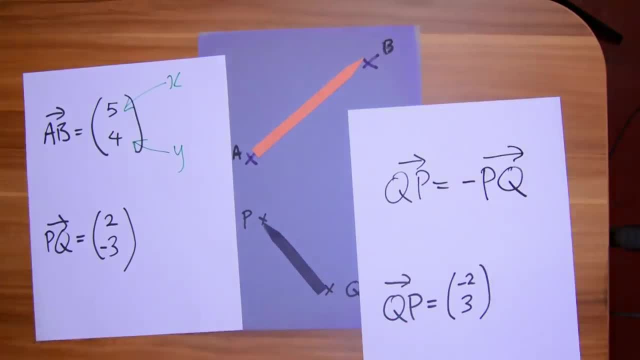 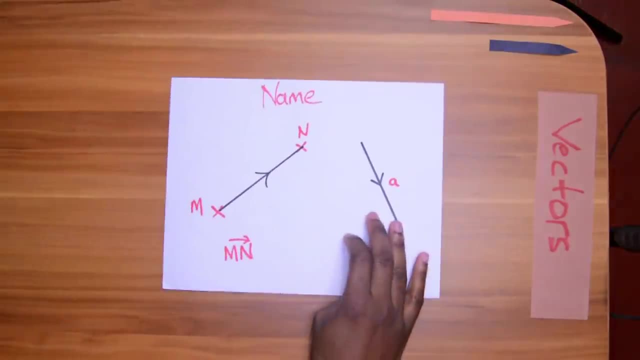 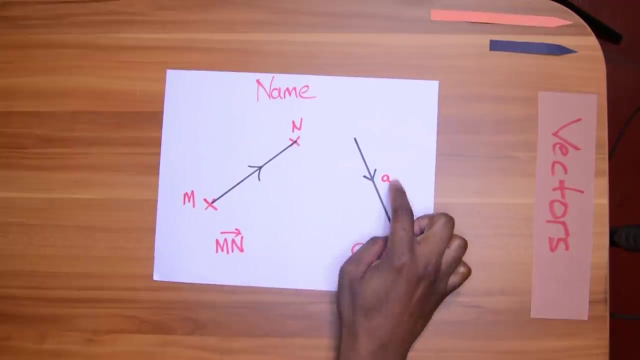 And that's a concept we use a lot in vectors. So what are some fun things we can do to vectors? Well, we can name them. This vector is named after the two points that it connects, so we'll call it MN. And this vector just has a nice, useful, one simple letter, and the letter must be common. 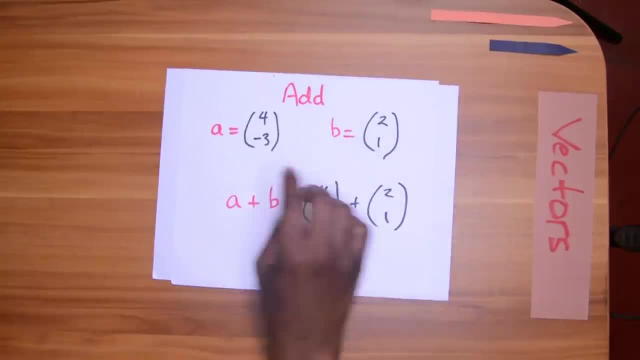 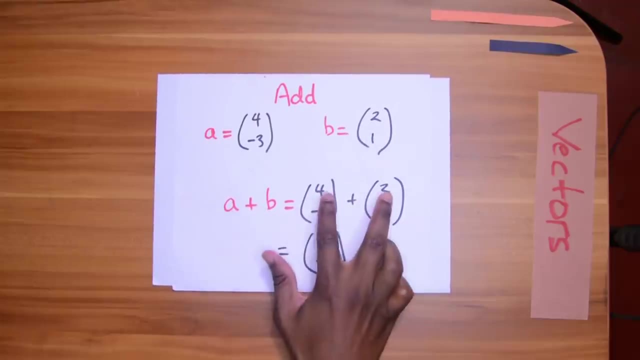 So this vector is called A. We can add them If we have a vector A and we set it to be 4, negative 3.. And vector B is 2, 1.. Adding A and B together, we'll add the X terms, then the Y terms and arrive at an answer. 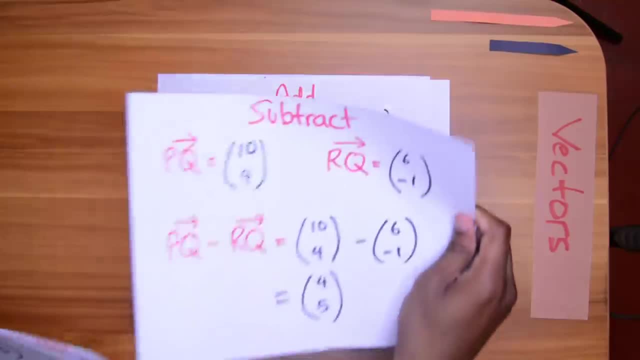 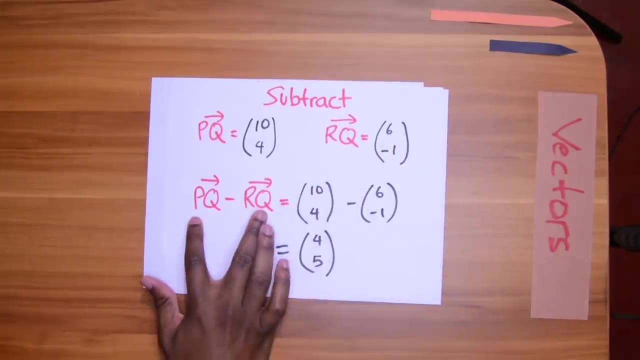 So this is the answer for A plus B. We can subtract them. Vector PQ is equal to 10, 4.. RQ is equal to 6,, negative 1.. If we subtract the vectors- very similar tradition- we use the X terms and the Y terms to arrive at our answer. 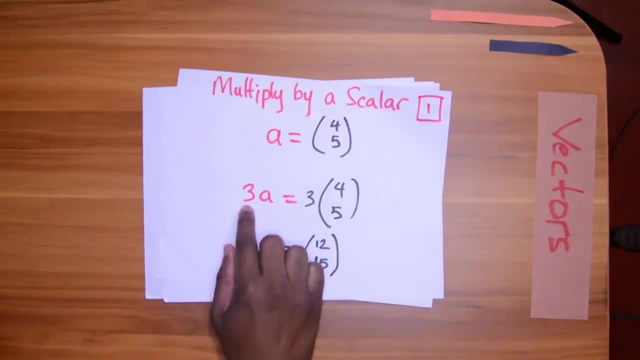 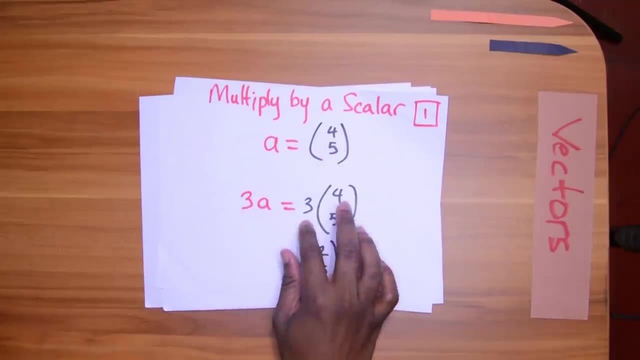 We can multiply them by a scalar. The scalar here is just this number. It represents a number. So when you see scalar you can think number A is set at 4, 5.. So 3A will be 3 times the X value, 3 times the Y value.